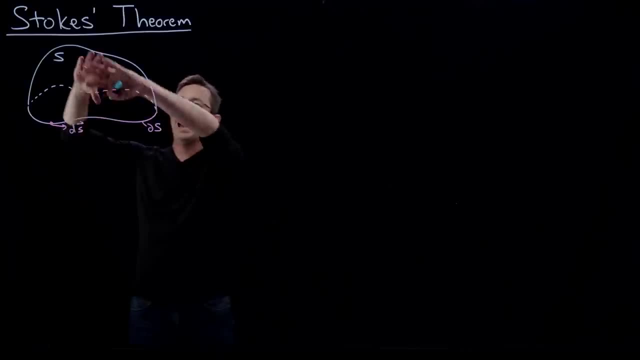 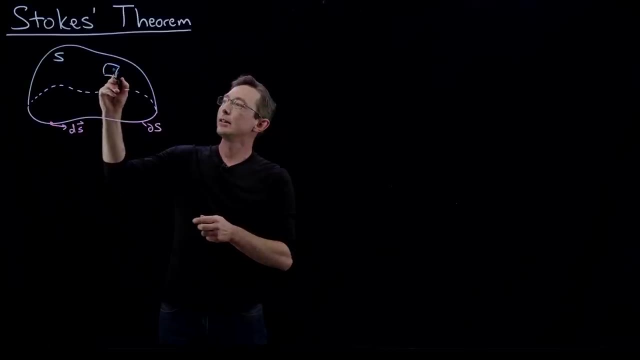 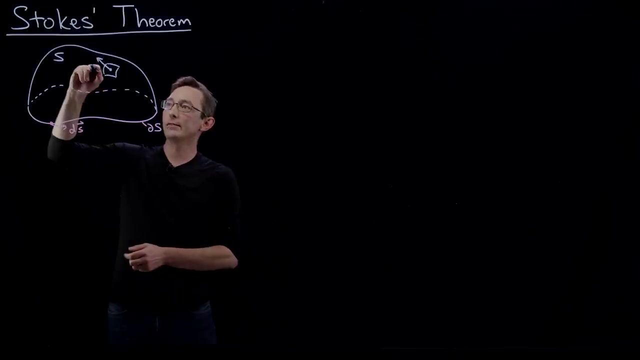 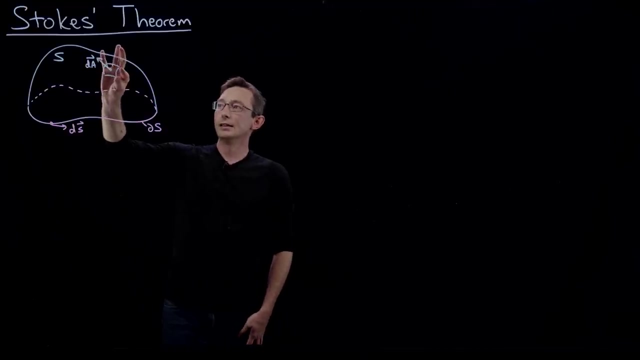 Okay. Similarly, at every patch on the surface s, every little kind of patch of s, there is going to be a vector in the normal direction, with area given by da, And so we're going to call this vector da. vector, Okay, Important, It has the magnitude of the area of that patch. 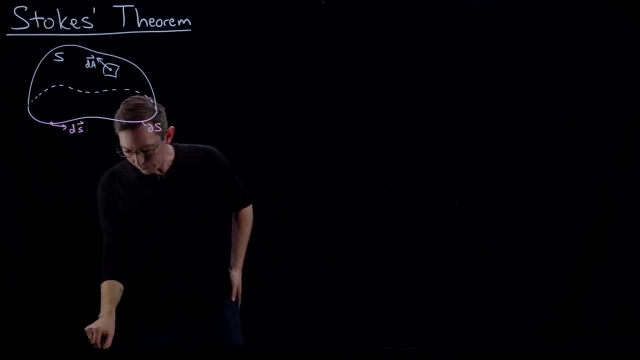 and it is pointing in the normal direction. This is important. Good, Now I'm going to write down Stokes' theorem in full generality And then, very quickly, I'm going to go to Green's theorem, because it's much easier to understand, kind of how things. 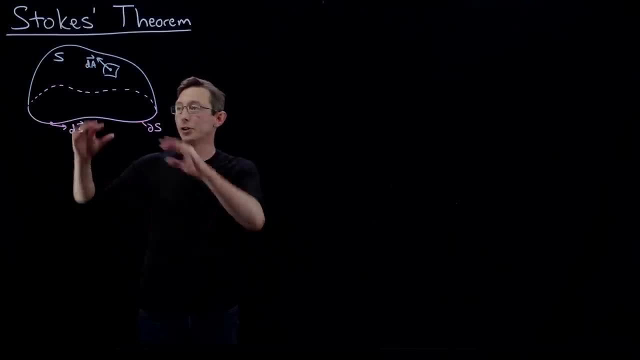 works. Green's theorem is like a 2D flat version, where, instead of a surface, we're just it's kind of a flat, flat surface and we are working on its perimeter. Okay, good. So Stokes' theorem here is- I'm going to write it as the integral around this entire surface. 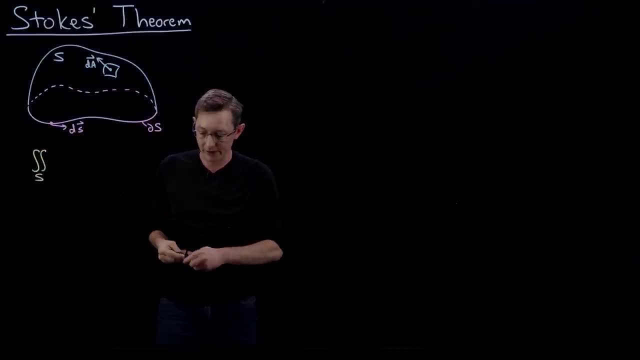 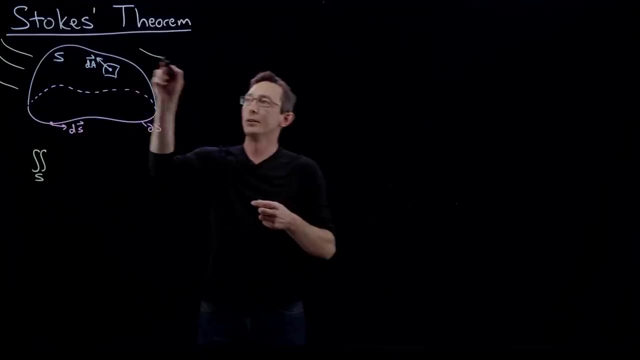 so the surface integral of the curl of some vector field, And of course I should always mention there is some ambient vector field. you know, kind of going through my volume, We're going to call this big F and it's going to have components F1,, F2, F3, just like it always does, And it's 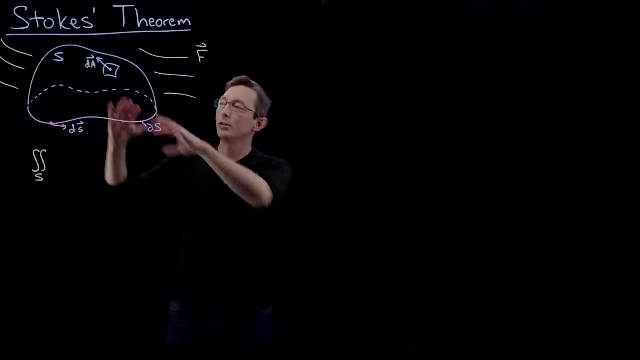 kind of passing through this volume And, if you like, you could also think of: maybe there's just a vector field on the surface of this volume, Maybe, maybe this is, you know, the northern hemisphere, And I have some vector field which is the, you know, atmospheric flow dynamics. 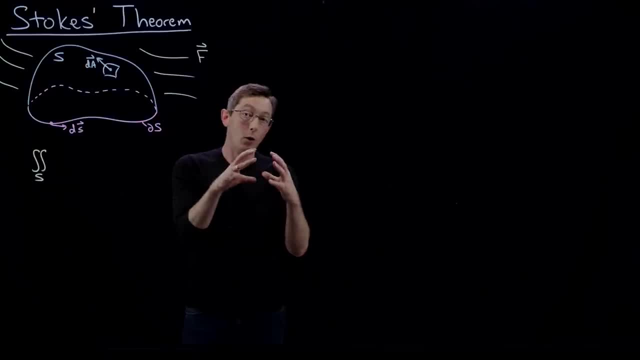 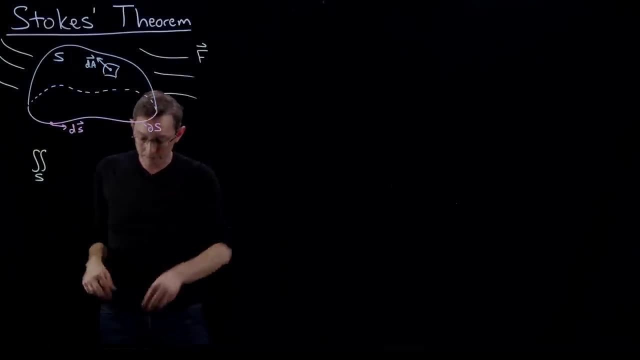 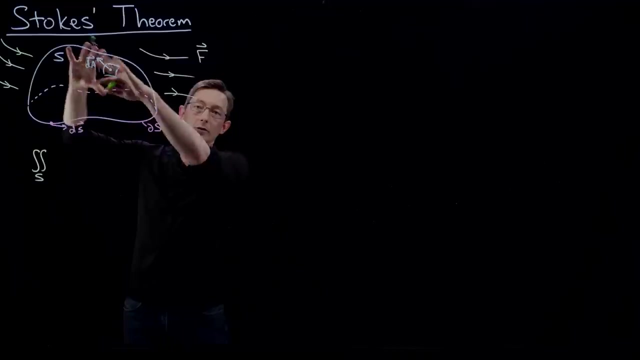 hurricanes and things on on that northern hemisphere. or you can think of an oil, you know, like a little bubble, a soap bubble. you can see the, the film, the vector field on the film. So there's some vector field F that is defined on the surface. It could be a three dimensional vector. 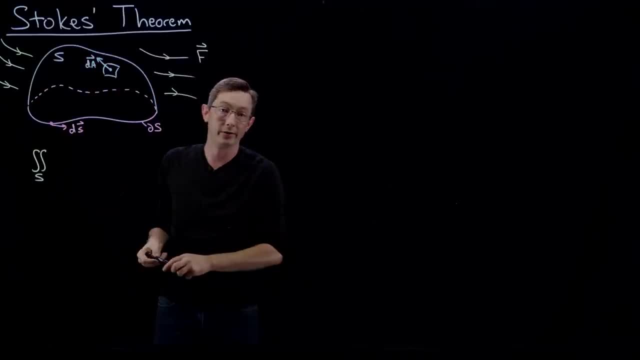 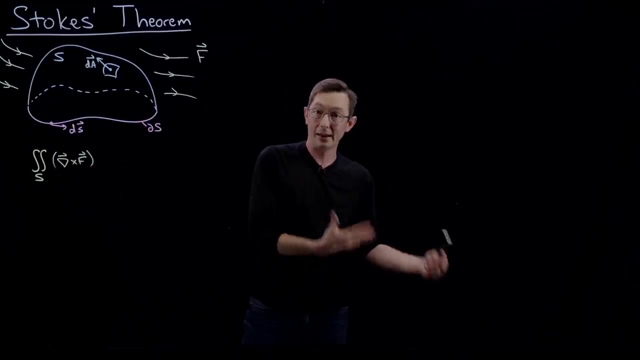 field and we just are looking at how it affects the surface. or it could be a vector field on the surface itself. take the surface integral of the curl of our vector field and remember the curl of a vector field itself is a vector field, so this is also a vector quantity. so essentially what i'm going to, 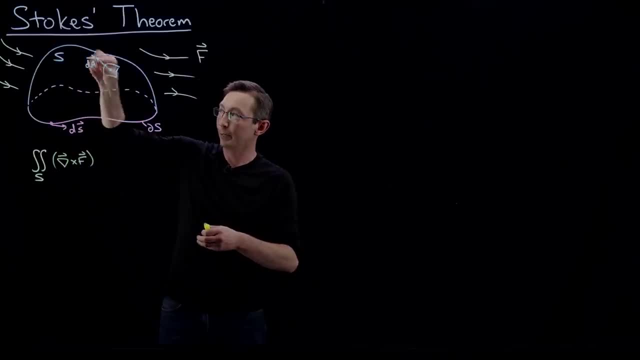 do is: i'm going to take my vector field. i'm going to compute the curl at every little patch here, every little patch. i'm going to compute the curl of my vector field and i'm going to integrate those up all along the the whole surface, and what i'm going to do is that curl should be pointing. 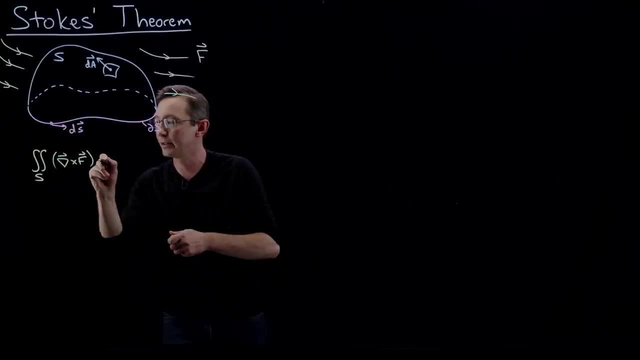 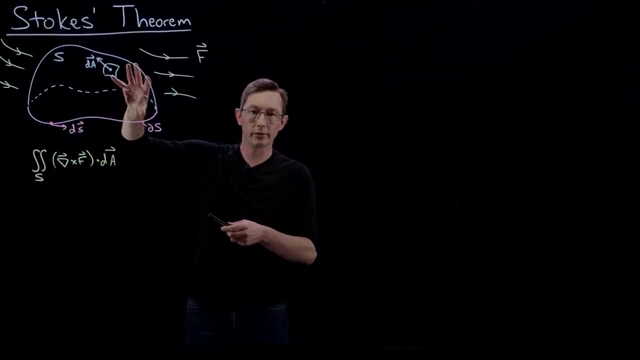 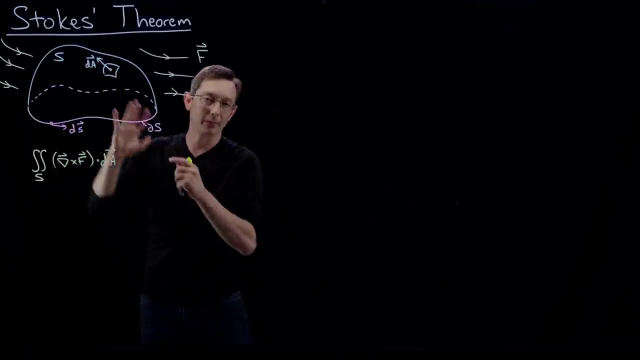 you know i want to see what is pointing normal to the surface. so i'm going to dot that with my d a vector. so this is kind of like integrating around the whole surface times d area. but because this is a vector field itself, i'm dotting it into the normal direction, okay, and i'll kind of give you. 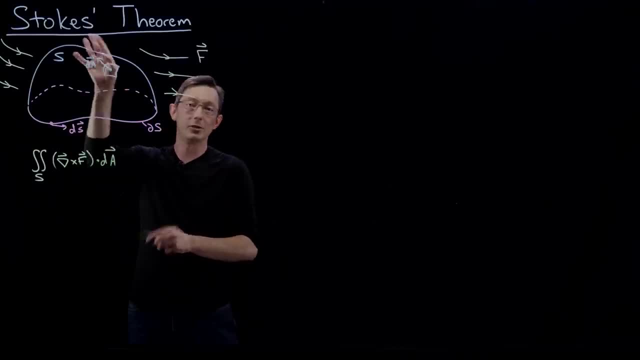 some intuition for why that's. that's we're doing this. this has a direction a little bit bit later, but anyway, we're trying to keep track of all of the curl. if we add up all of the curl of the vector field on the surface, what does that equal? sometimes i would care, like maybe the 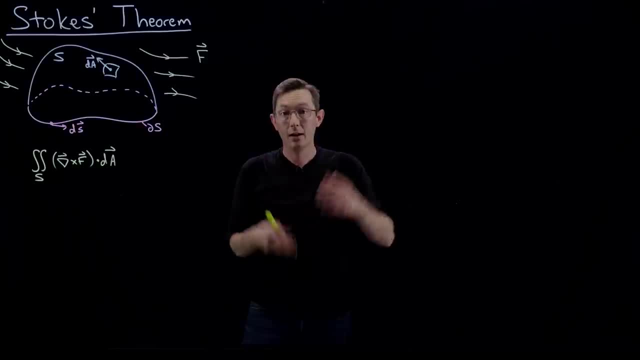 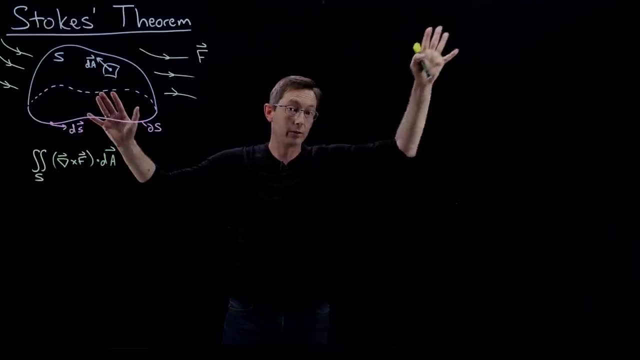 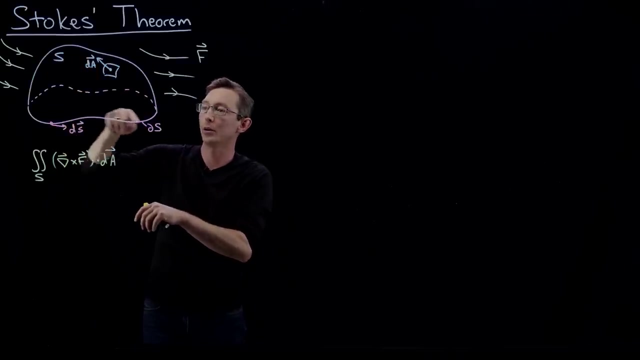 integral of the curl on that surface tells me how strong the hurricane is going to be, and that surface integral, just like gauss's theorem, allows us to take and equate volume integrals and surface integrals, stokes's theorem allows us to equate this surface integral to a path or a contour. 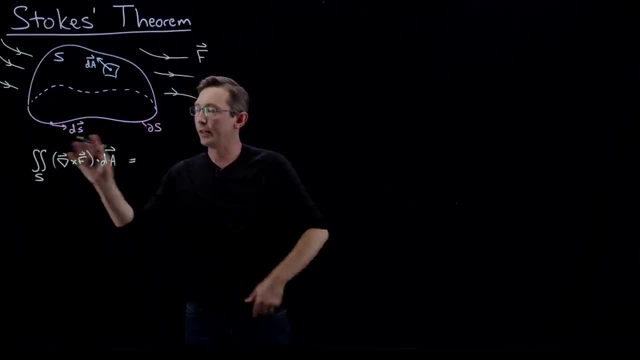 integral along this pink curve, and so, uh, the integral of my curl over the surface is equal to the integral around the perimeter on this pink curve of my vector field, f, dotted into this little tangential ds direction, this little ds, and so this is actually a really, really nice expression. this is a 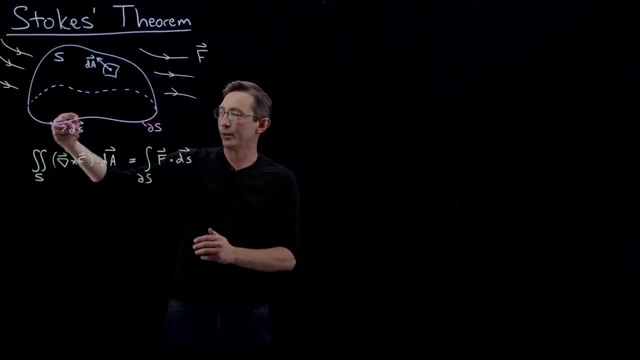 very easy to compute quantity. i literally just walk around this perimeter and i i take my f vector, my. maybe my vector field is pointing, i don't know. maybe my flow is pointing in that direction. that's f and i just dot f with ds and i keep track of how much of the f vector field is kind of in this tangent direction. 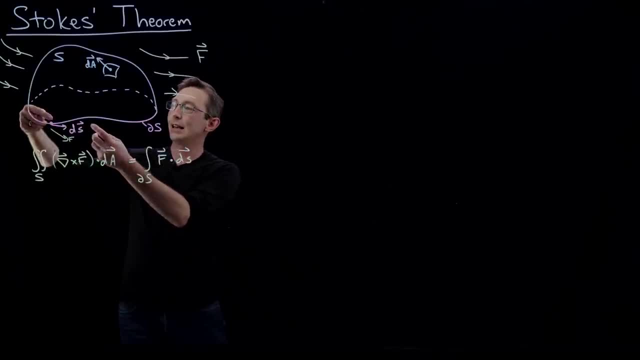 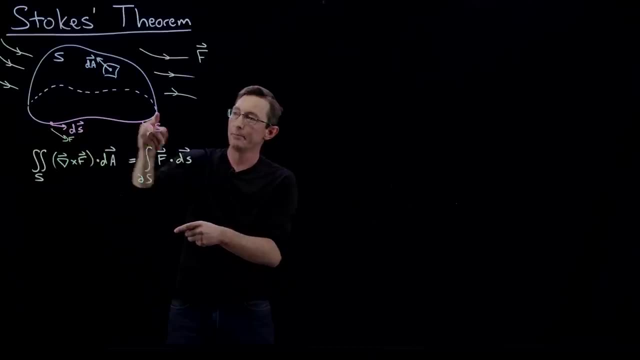 and if i add that up around this whole curve it basically says how much of f is kind of swirling around. if i am keeping track of the amount of f that's tangent, how much of that f is kind of in this tangential direction and that's a measure of the curl or the circulation kind of of the. 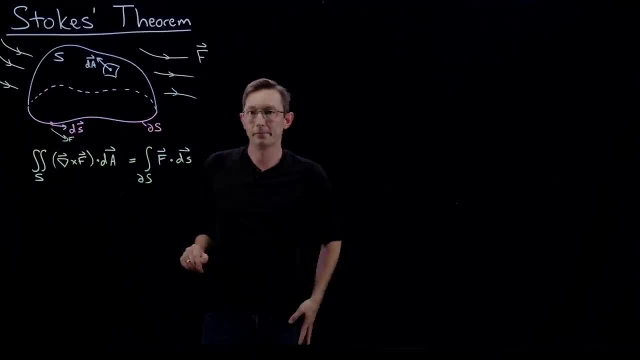 vector field on that perimeter. that's what, that's what this is and that's really remarkable that if i just keep track of how much my vector field is in this tangential direction, kind of over this closed orbit again, that tells me how much kind of like circulation or flow around this, uh, this. 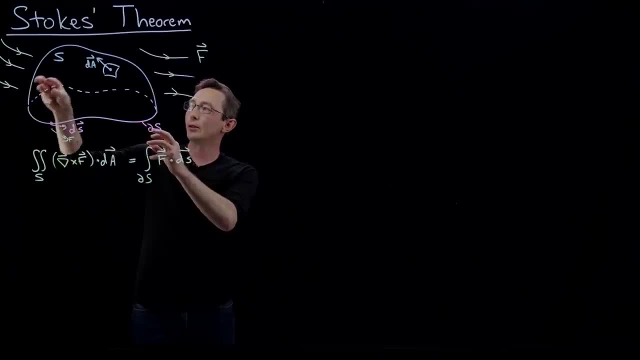 perimeter i have. that is equal to if i computed the curl at every patch on this circle of the surface and added all of those contributions up. so that's what stokes's theorem is saying, and it's a pretty remarkable theorem, okay, so, um, i want to show you how this works in green's theorem. 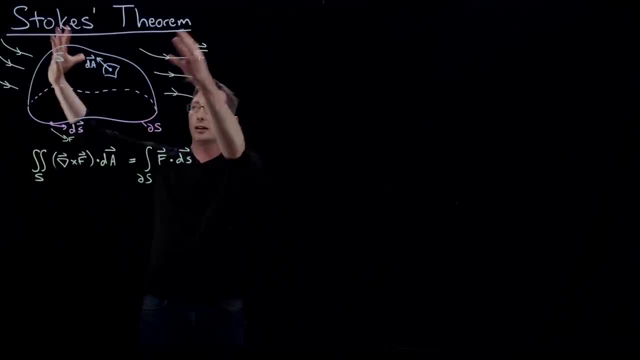 because i think it's really a lot easier to restrict this surface, to be flat, and look at green's theorem. so that's exactly what green's theorem is. so green's theorem is essentially stokes on a flat surface s okay. so what we're going to do is we're going to look at kind of a top down. 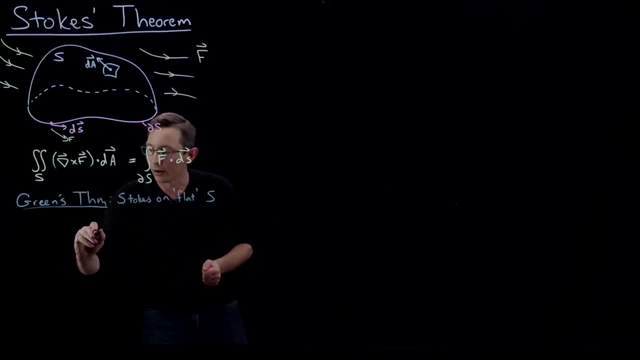 version of this where now we have our our surface s, we still have our perimeter partial s, and essentially what we're going to do is write this expression here. but uh, looking at this 2d flat surface, so now my surface is flat and we're going to do the exact same thing and i'm still 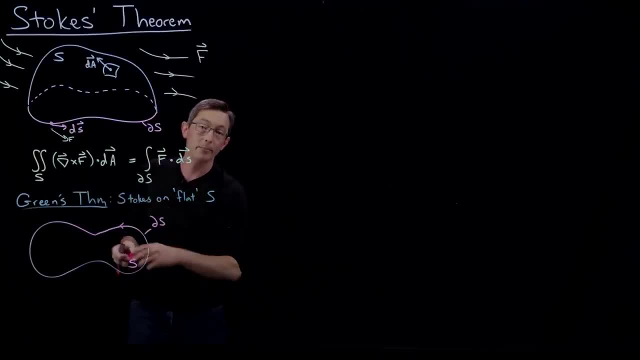 orienting this curve so that it moves in the, i believe, counterclockwise orientation. okay, that conforms to the right hand rule. so we consider this kind of the positive direction along that that perimeter. okay, good now green's theorem is is exactly stokes's theorem, restricted to- uh, to a flat. 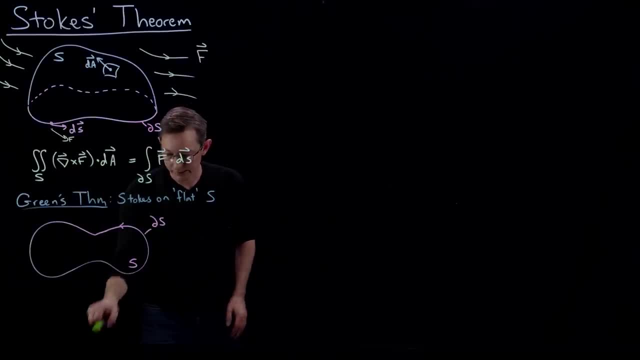 surface and we can write it down pretty simply. so i'm going to write this down and we're going to say now that our our f here, f in 2d, just has two components, f1 and f2, and any curl that i have if my vector field is doing some. 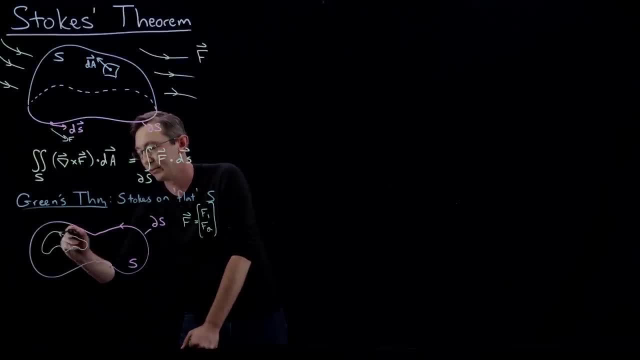 you know, maybe it's doing some swirly things like this. i have some some kind of like circulation components, you know doing some circulation. then, uh, the curl is going to be pointing out of the board. so any positive curl is going to be in the kind of k or z out of the board direction. okay, so 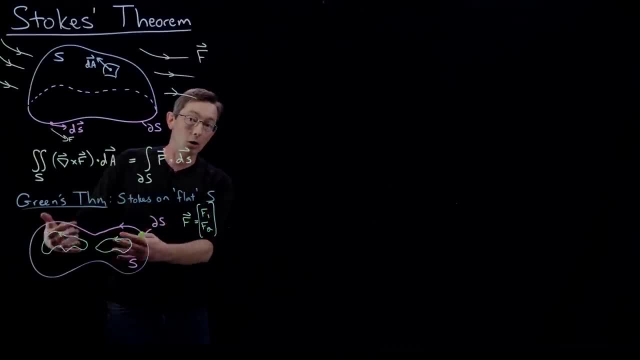 that's why it also helps to think about this in 2d, because all of the curl is in the kind of out of plane third component. and so green's theorem or stokes's theorem on this 2d slice essentially simplifies to this surface integral. so this integral over s of the curl of my vector field, 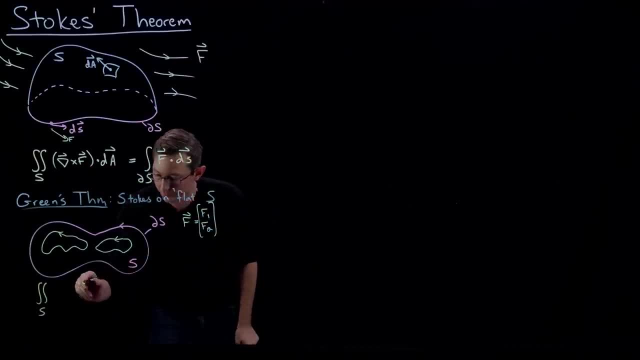 now the curl of a 2d vector field is just partial f 2, partial x, minus partial f1, partial y. and now, if I think about it, every little area patch, the normal, is already in the Z direction. so I just have to multiply this by the. 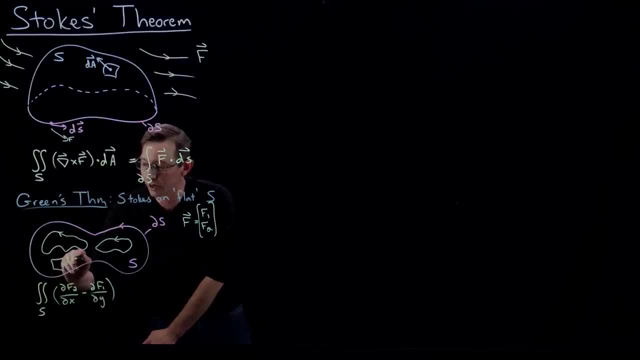 little D D area patch here which is DX times dy. okay, so this is a simpler expression for this, this integral of the curl. here I'm just integrating up the curl of this 2d vector field over this entire surface and Green's theorem says that this is equal to. again, it's equal to my vector field F, dotted into the. 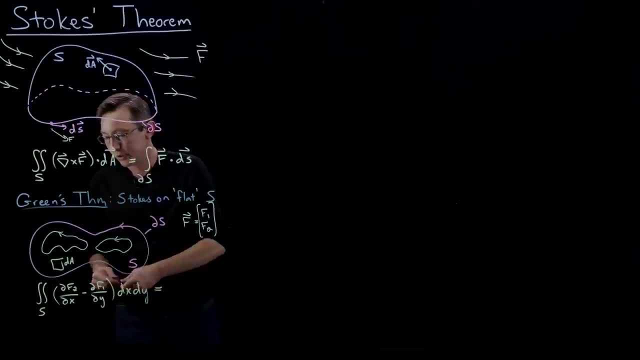 tangential direction into this little tangent direction. so if I take, you know, if I have this little DS vector and I have my F vector, I just go along the perimeter adding up how much. what is F dotted with DS? okay, and so the nice thing is is that this is an integral around the perimeter of F. 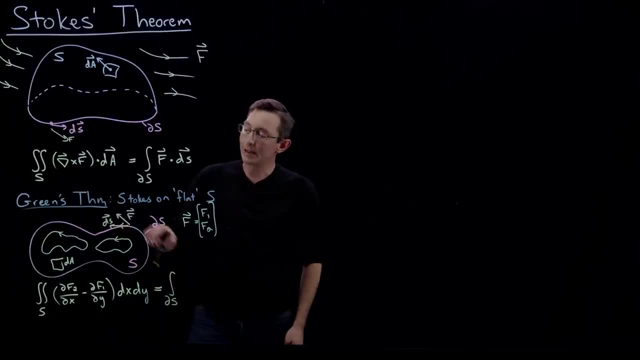 dotted into the tangential direction, but because I'm already moving around a this, this curve, that's, that's parameterizing the perimeter. this is essentially just F, 1, DX plus F, 2, dy. okay, so I literally take how much of F, how much of F1 of the F1 component is in the DX direction of this little sorry. 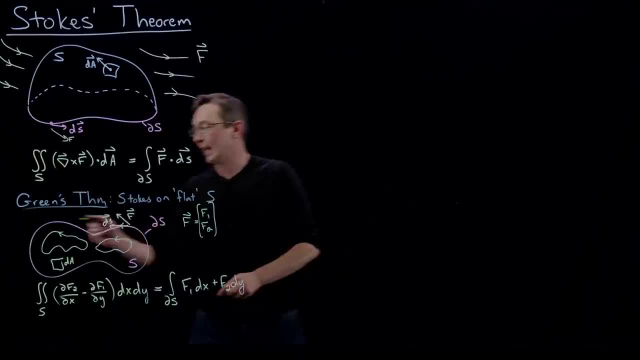 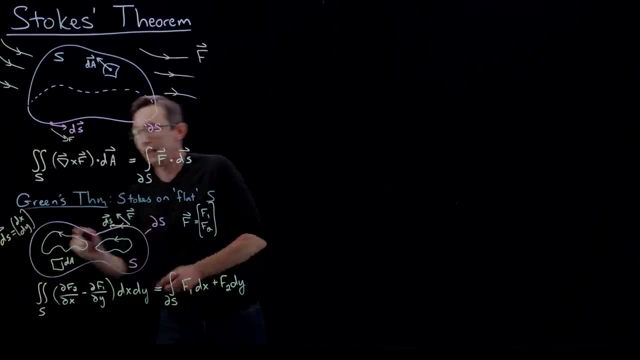 I'm getting ahead of myself. let me slow down this little d-s vector. d-s vector is equal to DX dy. it tells me at every little point here: is my vector moving more in the DX direction or the D? y direction. it tells me what the the. 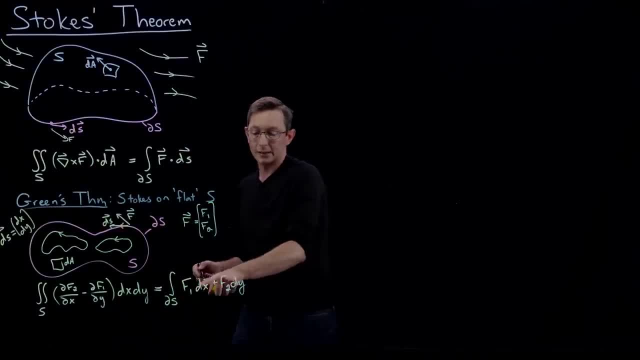 direction of my curve is D, X, D, Y. those are the DX and these are days right now. those are the dx and dy here. okay, and we integrate all of those little dx's and dy's along this surface. so this is green's theorem, and again it tells us that i can basically just walk around. 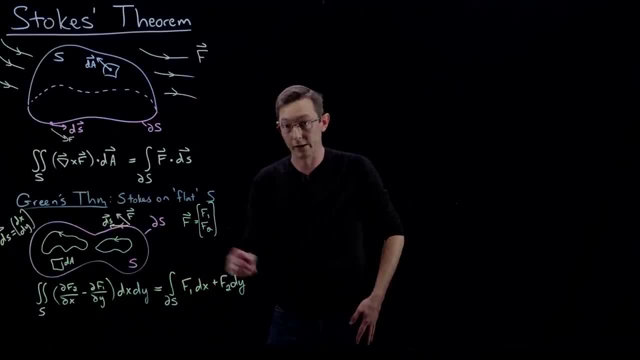 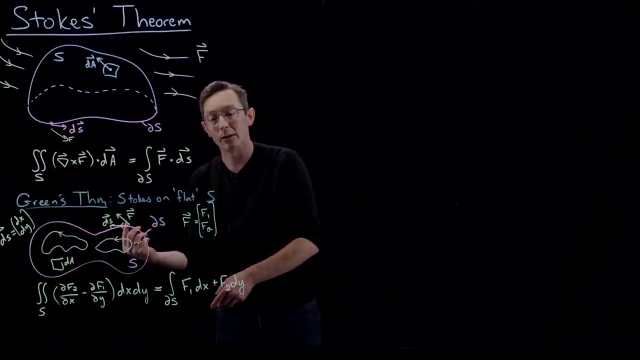 along the perimeter of this vector field. adding up this quantity, just literally, taking f1 dotted into the dx component of this tangent vector, plus f2 dotted into the dy component of this tangent vector, and if i add up that number around this entire perimeter, it equals the sum of all of the. 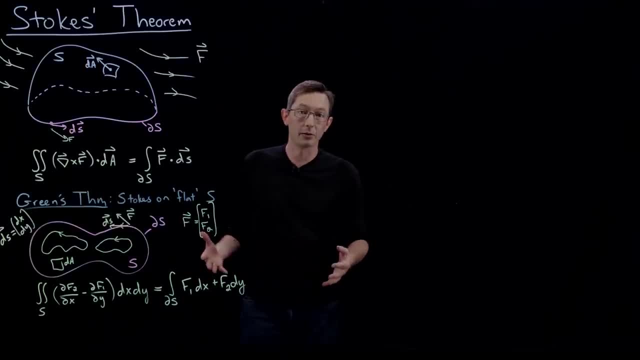 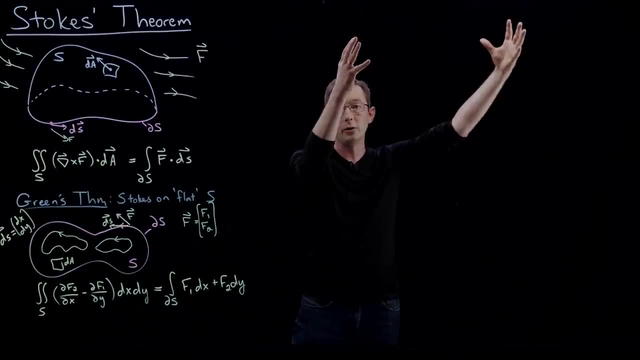 curl of my vector field on the entire surface, uh surface integral. so again, this is a lot like gauss's divergence theorem where we're going from a big integral, you know, over a volume, down to a smaller integral over a surface area. here we're going from a big integral on a surface down to 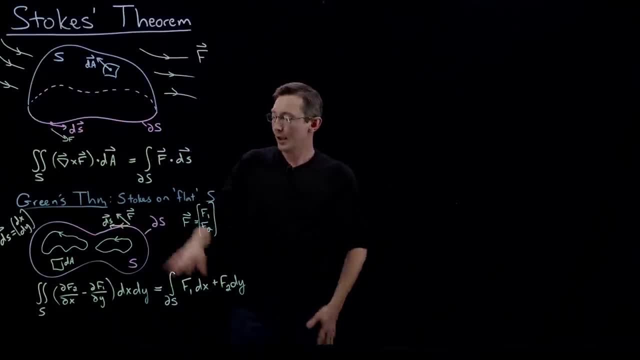 a smaller integral on the perimeter of that surface and the same thing here. so here's a couple things i want to do. i want to give you some physical intuition for why stokes's theorem and and green's theorem are true, and then i'll tell you some cool examples of these. okay, 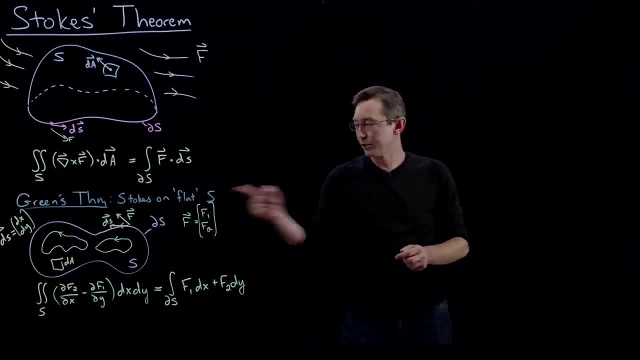 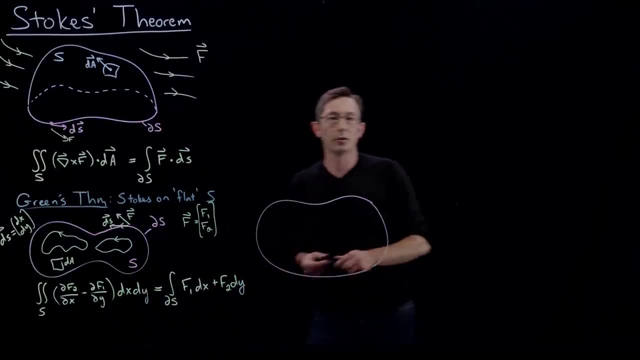 so, um, maybe the first thing i'll do is i'll just draw this picture again and we're going to do the same kind of pillbox, uh decomposition that we did before for, uh, for gauss's theorem. so what we're going to do is break this up into a number of little boxes. so i have a number of little boxes. 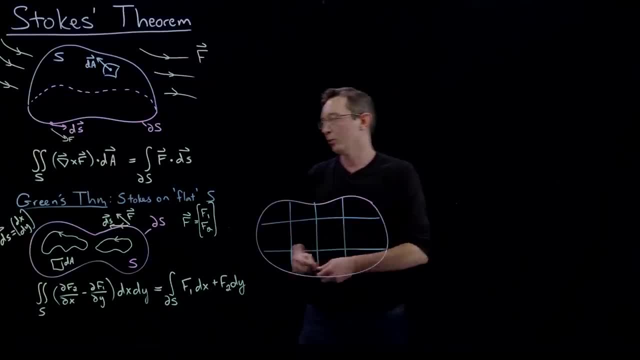 i have my kind of kidney bean uh shape here for for the the surface, and we're going to break it up into a bunch of little boxes. now i've only drawn, you know, 12 boxes here, but in what we're going to do is essentially imagine we take the limit as these boxes get infinitesimally small and 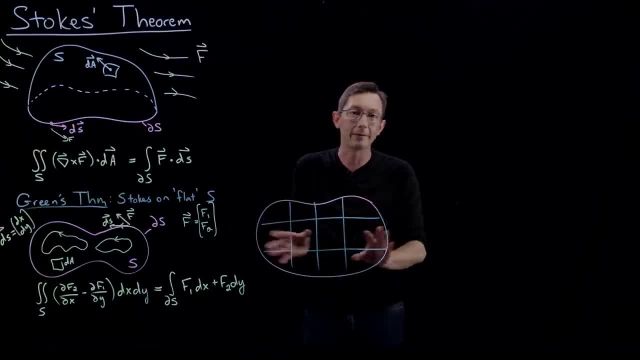 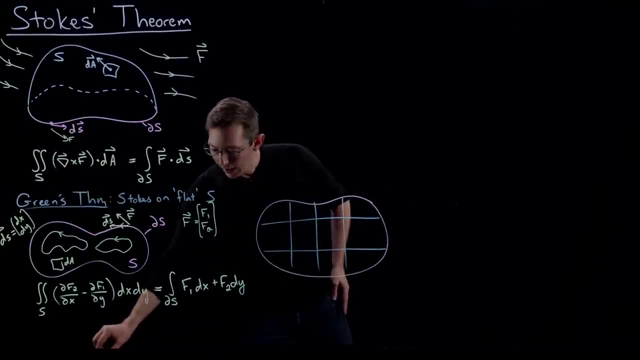 infinitesimally close together. so this is going to be a really, really finely resolved graph paper kind of uh, representing this, this area, and so what we can do is essentially look at the curl in every little box here, so the little local curl in every little. 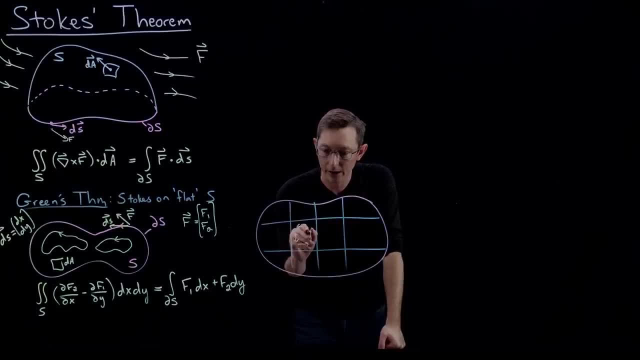 box is kind of a little vector field that's going around in a circle. this is a little positive curl, uh representation here, and the next thing is going to have a little curl. these are all going to have, you know, a little bit of curl and i'm just going to draw these, um, and just like gauss's divergence. 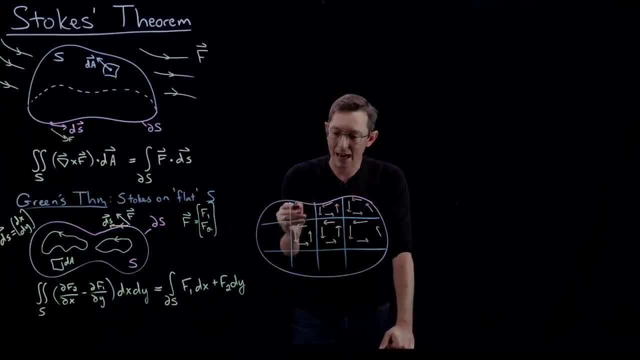 theorem you can already start to see. uh, what i'm going to do is i'm going to draw these of these little little circles that i've drawn for each of these little circles, and what's to do is i'm going to move these to a new surface and, of course, what's going to happen is that 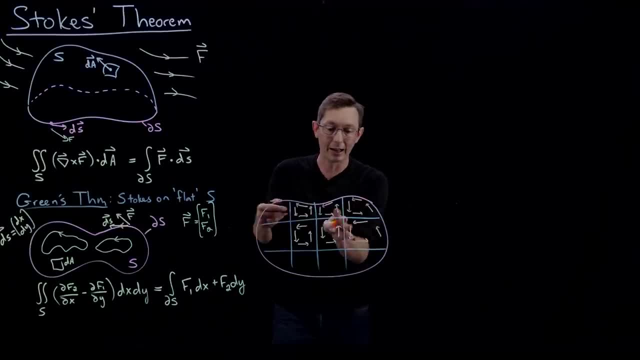 the inner cells, the curl from the neighbors are going to cancel each other out, and so if i integrate all of these curls over the entire area, all of the inner kind of components of the curl are going to cancel out to zero and i'm only going to be left with the component that's kind of in this tangent direction around the perimeter, and so that's the real idea here. maybe i don't have to draw the the whole thing, but i think you get the. 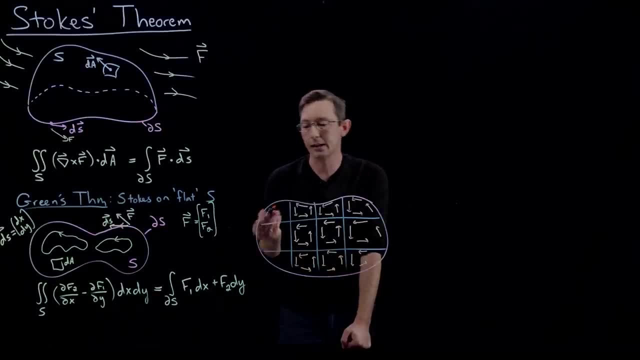 the idea, hopefully, that, just like Gauss's divergence theorem, if we have these infinitesimal little boxes and if we assume that our vector field is sufficiently smooth that these are continuously varying from cell to cell, so if f is a smooth vector field and most of the vector 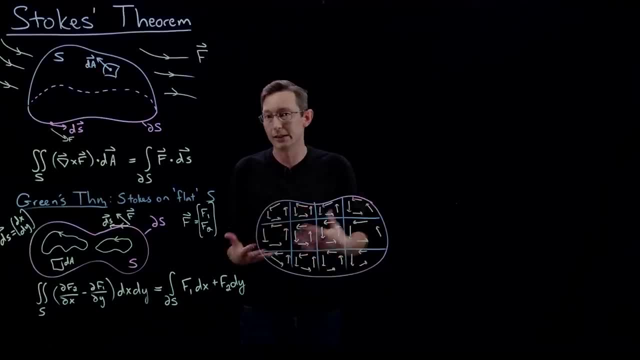 fields I think about are smooth. Fluid flows are smooth typically, except for shock waves. The flow over a soap film is smooth and continuous, and so that basically means that these different kind of components on these different edges are canceling each other out. 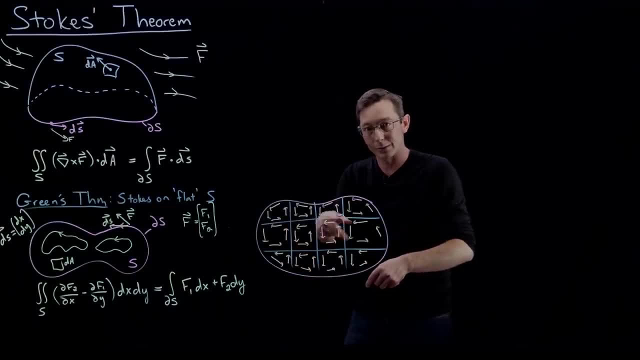 This little box is swirling a tiny little vortex. this little box is swirling a tiny little vortex, and the up component and down component cancel each other out on every single inner wall here, and so all that's left are the little components that are kind of in this tangent direction here. 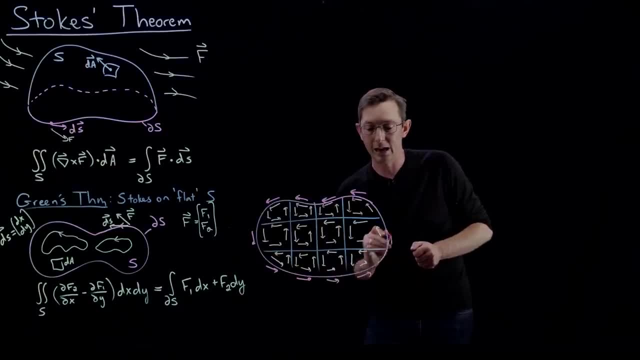 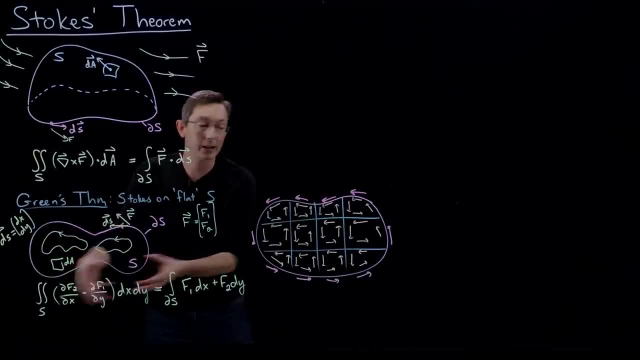 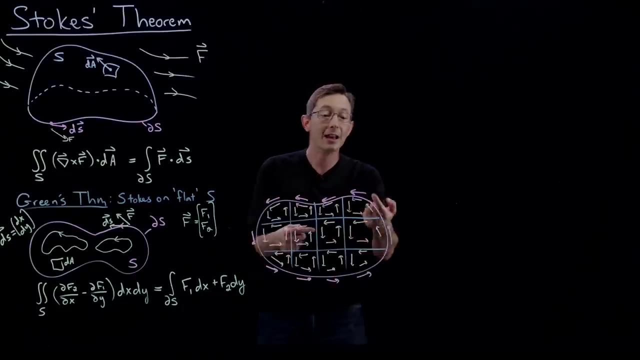 that are kind of aligned with the tangent of the perimeter, and so hopefully that gives you at least some intuition for why the surface area of the curl is equal to a path integral of the vector field dotted into the tangential direction, the tangent component, the component of the vector. 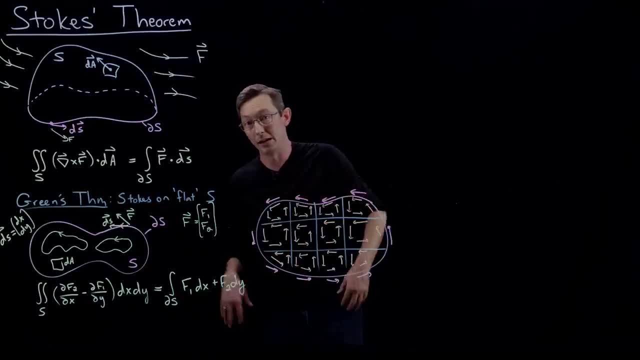 field that is tangent to this, enclosing pink perimeter. Okay, so that is at least the cartoon of why Green's theorem is so important, and so I'm going to go ahead and show you a little bit more about why Green's theorem is true, and Stokes' theorem is just kind of a more general case of. 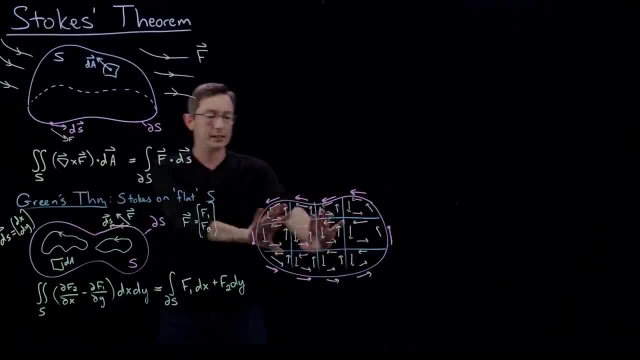 Green's theorem, where you now take this two-dimensional surface and you imagine that there is some three-dimensional surface over this perimeter, and the same basic argument applies If I grid this up into little boxes and I look at all the little curl components, all of the inner. 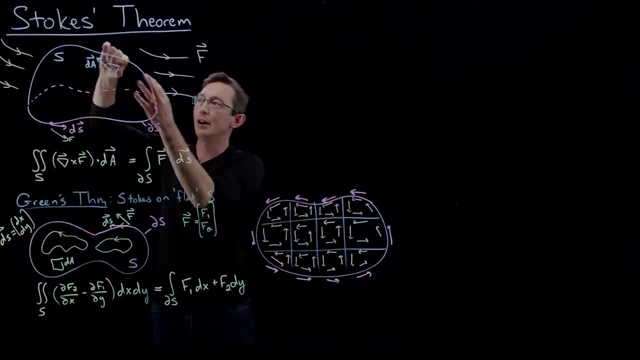 kind of inner walls are going to cancel out, and the only component that's going to be left when I integrate over this entire blue surface area is the part of the vector field that is tangent to this pink perimeter curve. So again, the integral of the curl of F over this entire surface is 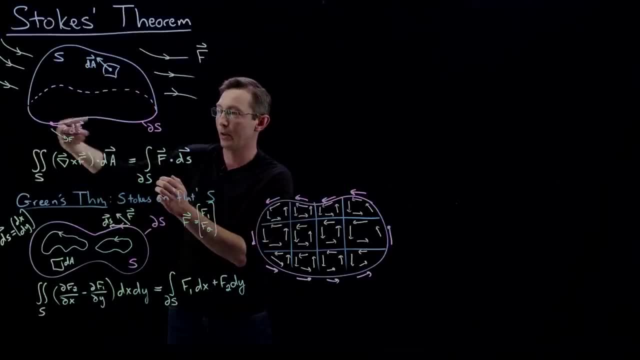 going to equal the integral over the little contour, the perimeter of my vector field, dotted into the tangent direction just the tangential component, And this is really cool If we think about you know, let's say we're talking about planet Earth and so we have. 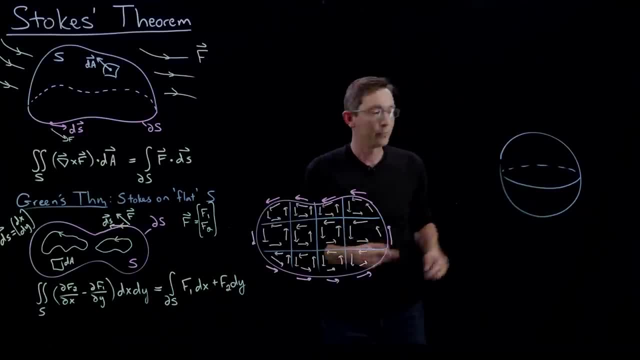 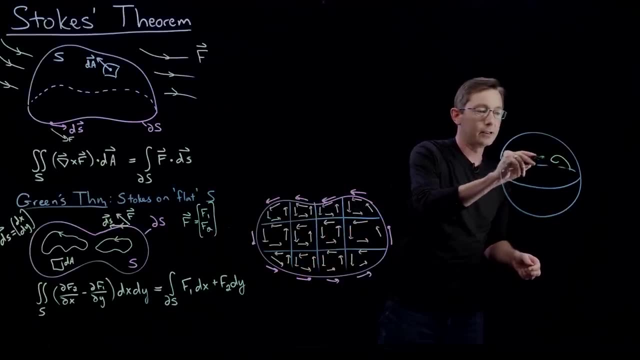 you know we're going to look at the, the northern hemisphere here and let's say I have a big. you know I'm not sure I can draw a big hurricane, but let's say I have, you know, some, some big hurricane forming in the northern hemisphere. If I added up all of the curl of every little patch on this northern hemisphere. 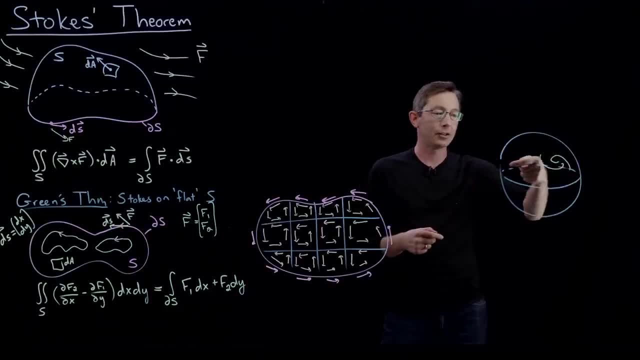 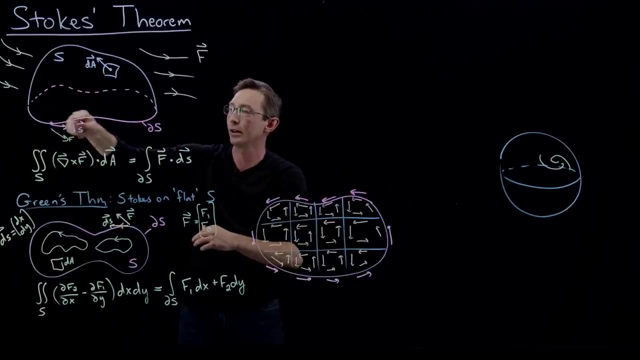 that would equal to the amount of the vector field integrated along this perimeter, dotted into the tangent direction. And so you can think about it: if this, if this surface, if this vector field is swirling, you know, around in the surface, there will be a signature of that swirling on this pink perimeter here and we'll be able to compute. 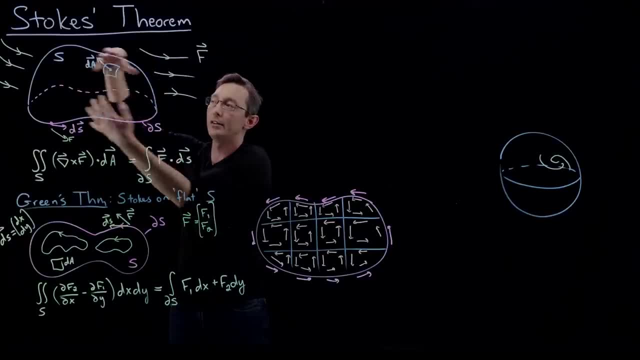 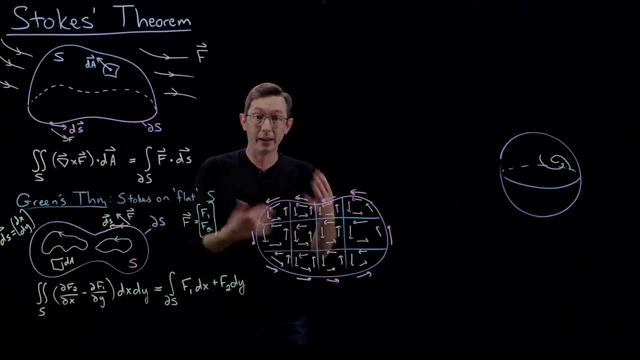 kind of how much circulation or vorticity there is in the surface, just by computing what is the accumulated amount of circulation on this, this perimeter here. So it's a really powerful idea and this is going to be useful for things like fluid flows, where we have circulation and rotation. 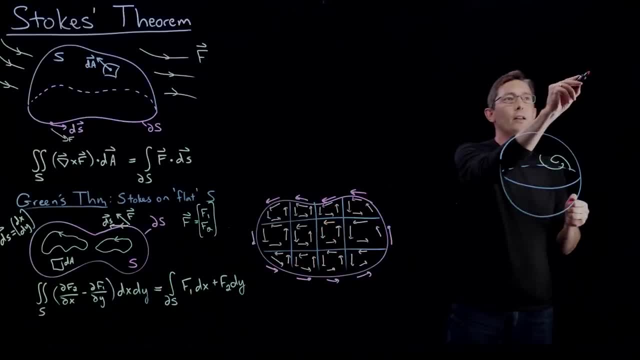 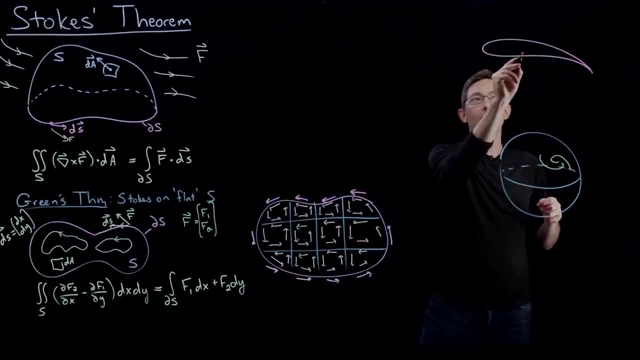 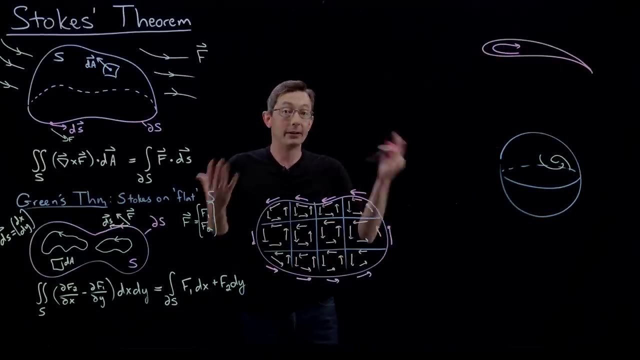 So this is actually really useful when we think about airfoil theory. So if I have a wing, I might want to compute kind of how much, what is the circulation of flow kind of over that wing, and that will be relevant for computing the lift over the wing, things like that. 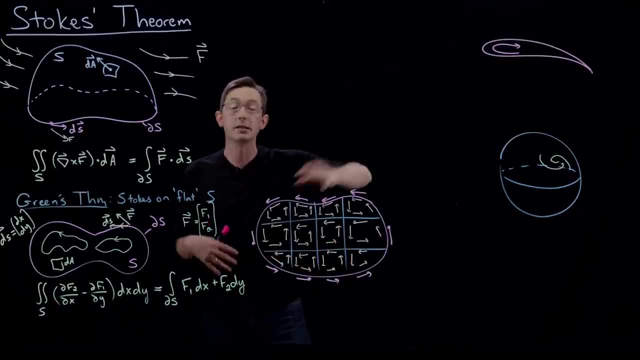 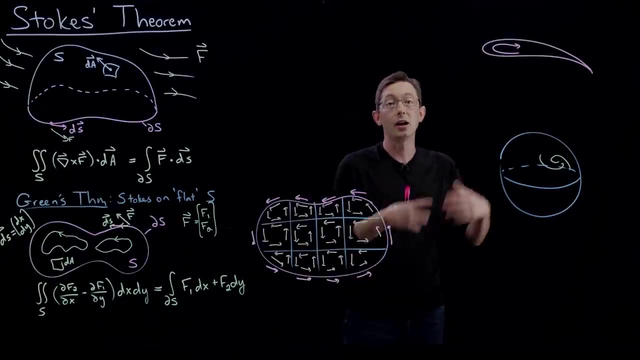 So you know, curl and Stokes' theorem are really important when we think about aerodynamic surfaces and fluid flows over aerodynamic surfaces, hurricanes, things like that. And this is going to be how. remember, divergence theorem is how we encoded conservation of mass, conservation of momentum, into Navier-Stokes equations. 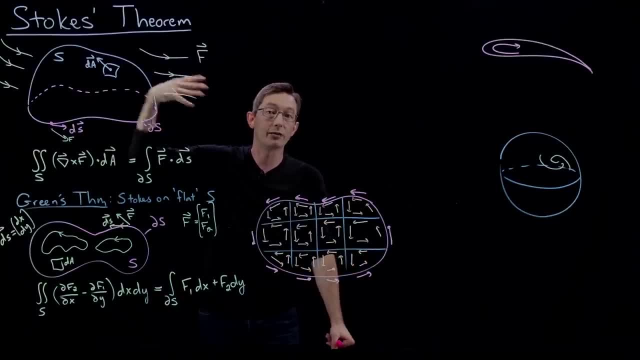 Stokes' theorem is how we're going to encode conservation of angular momentum. So all of this curl is kind of measuring how much angular momentum I have, and if I add up all of that angular momentum there's a signature of it in the perimeter of that surface. So really really powerful idea here. 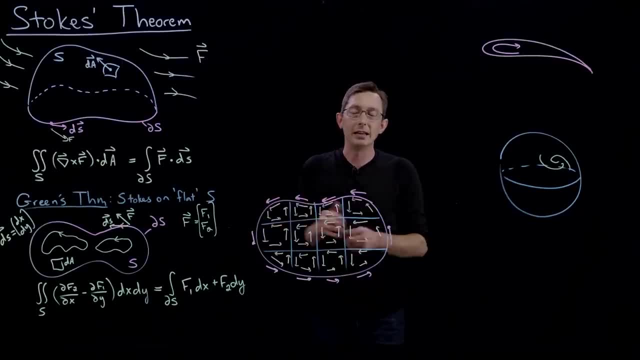 And one last thing I'll point out, and this is just something neat. I remember one of my favorite calculus teachers in high school taught us this, and I think it's a really cool idea. You can also use Green's theorem or Stokes' theorem. 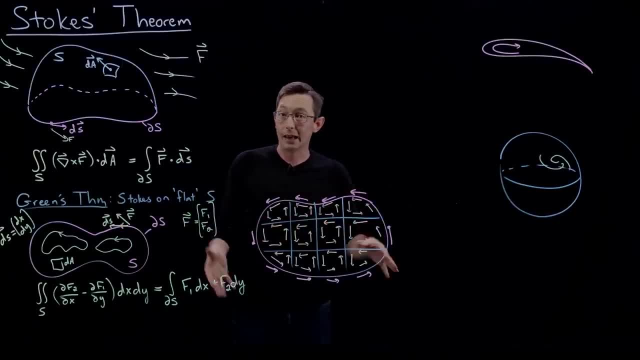 to compute the area of a tract of land. So back before GPS, back before, you could just kind of use satellites and GPS to compute the area of an irregular shape of land, or use a computer program. surveyors would actually have to walk around the 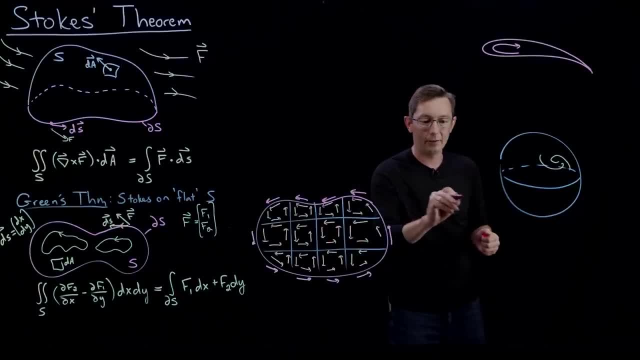 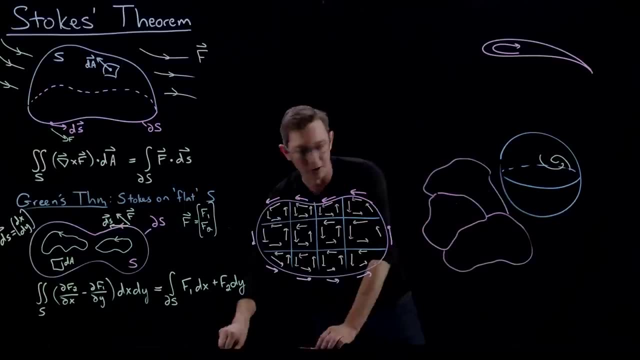 boundaries of someone's property. So maybe I have a farm here and I have another farm here and I have another piece of land here and maybe there's a river, you know that's going, you know, on the boundary of these. 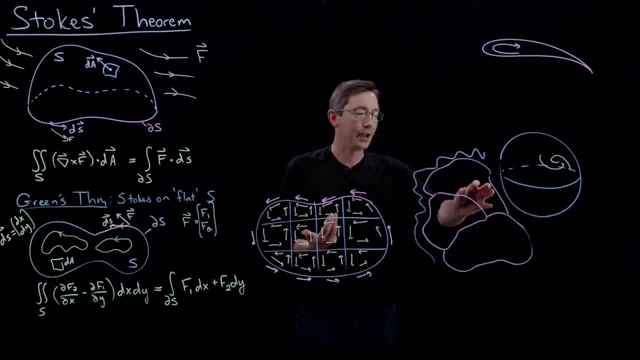 How do I compute the area? you know how many acres or how many hectares of land are inside this area. if I want to sell a parcel of land and it's got an irregular boundary, Well, it turns out you can use Stokes' theorem for this in a real 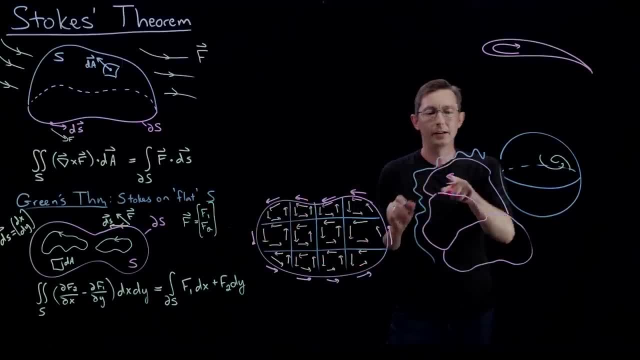 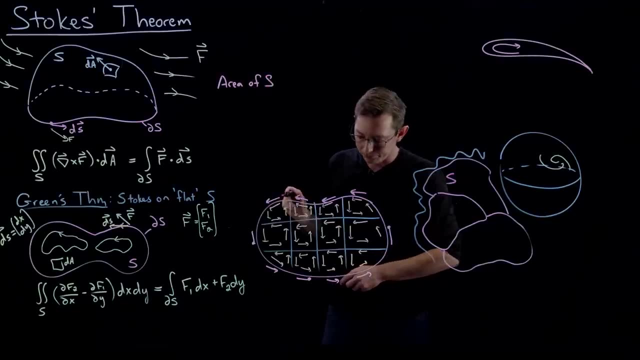 really clever way. So let's say I pick, you know, one of these areas here, S, one of these irregular shapes, S. Then the area of S is equal to one-half times the integral around its perimeter. around the perimeter of S of 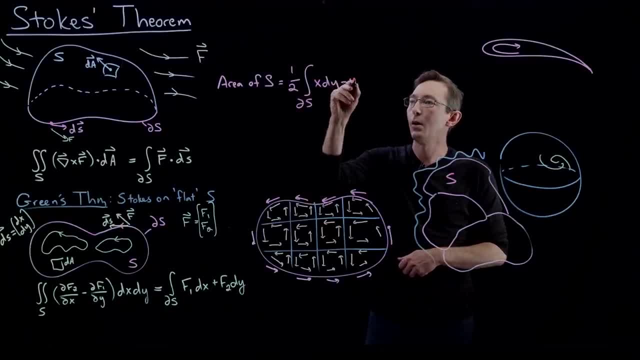 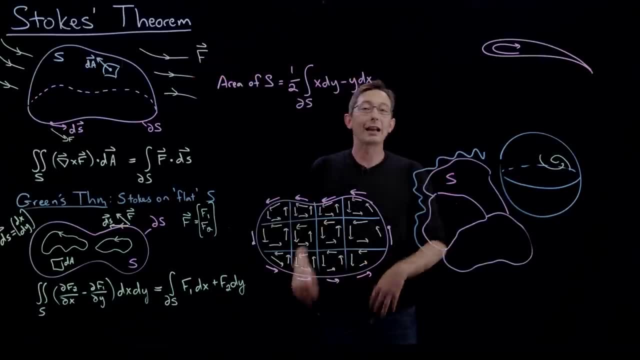 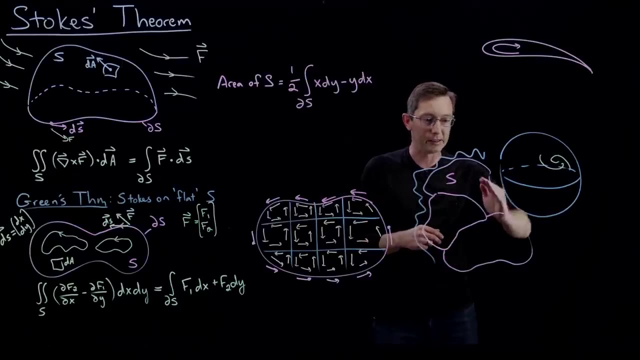 x dy minus y dx, And I'll tell you why this is true. So this is true, And so what I can literally do is I can walk around, I can go. you know, I bring an apple and a nice book and I'm walking around this perimeter and I literally count. 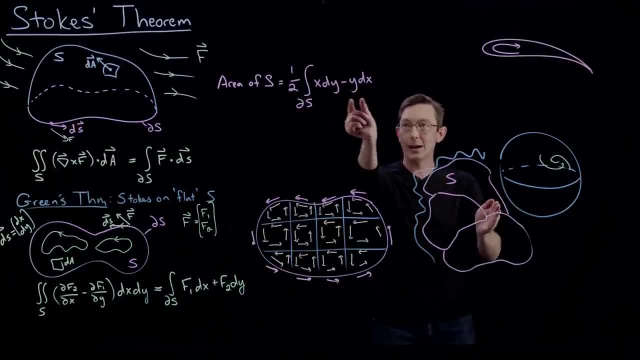 you know how many times I step in the dy direction versus how many times I step in the dx direction as I go along this perimeter and I add them up in this formula. So I literally, as I walk around this perimeter, I compute this quantity and when I come back to my starting point, 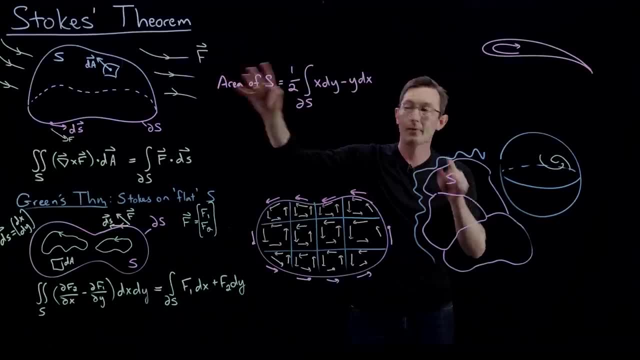 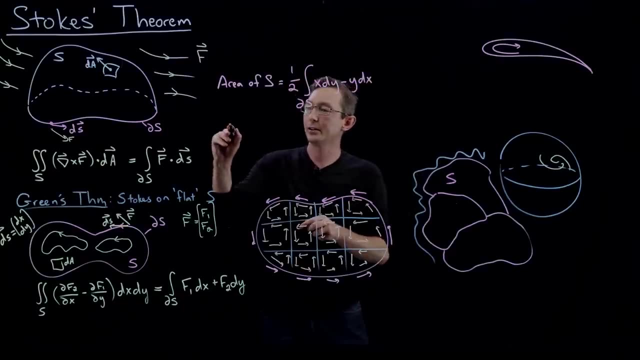 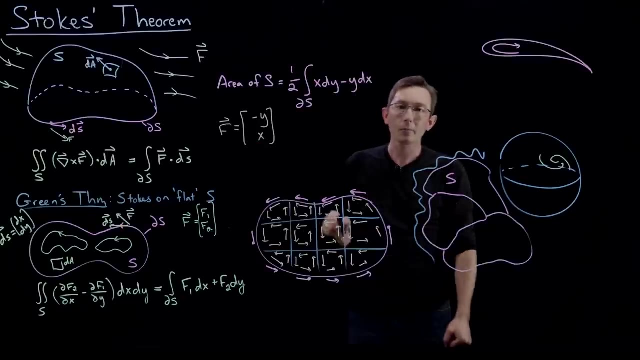 I will have swept out the area of S. Now, why is this true? This is true specifically because our vector field, here, this corresponds to a vector f that equals minus y, x, And so, if I think about it, the curl of this vector field, so the curl of f. 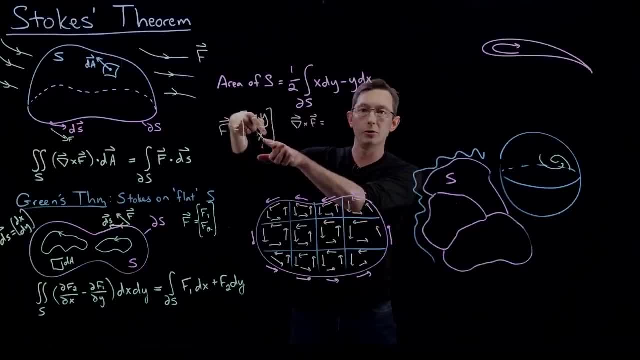 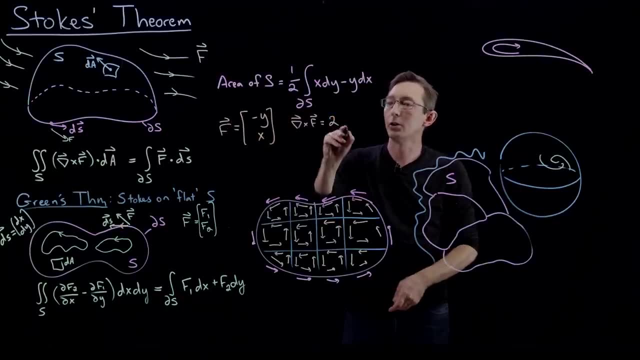 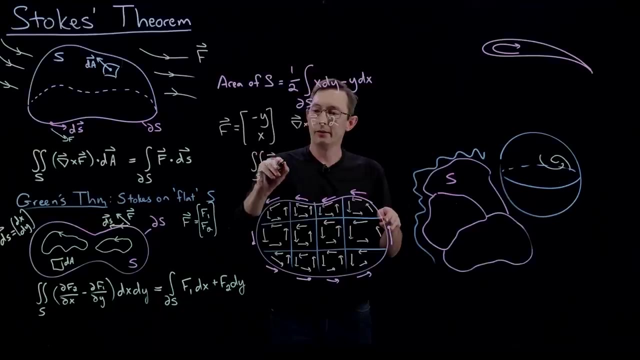 is equal to partial of f2 with respect to x, that's 1, minus partial of f1 with respect to y, that's minus minus 1.. So this curl equals 2.. So if I do a surface integral over S of the curl of my vector field dA, that should equal. 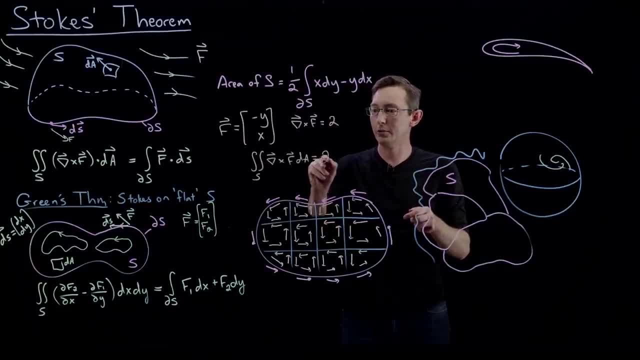 2 times my area, 2 times this area. let's call it A. okay, But I don't want to actually break this up into a bunch of little surface areas. I don't want to actually parcel this out. I want to actually parcel this out to measure the area. 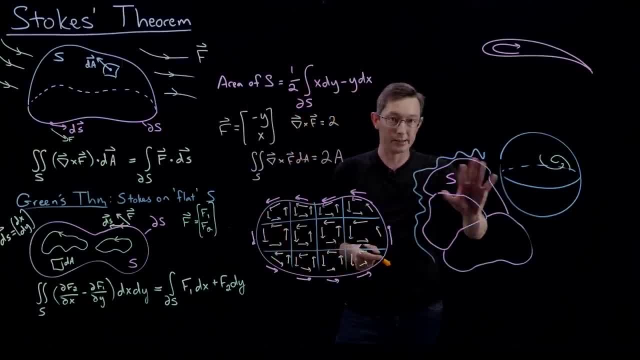 So we're going to use Stokes's theorem, or equivalently Green's theorem- because this is a flat surface- to instead integrate around the perimeter. So this is equivalent to the same integral around the perimeter of my vector field f, dotted in the perimeter tangent direction. 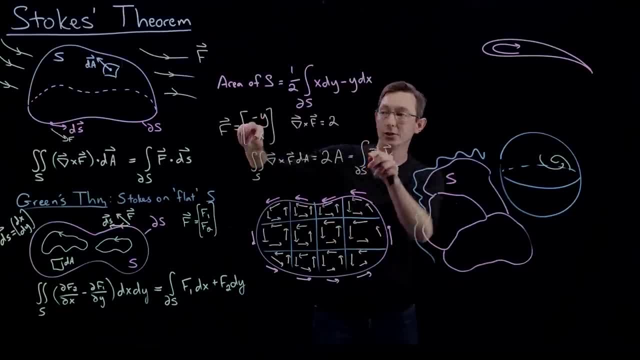 And again f dotted into the perimeter tangent is minus y x. Minus y in the dx direction, plus x in the dy direction. That's what this quantity is, And so if I just integrate this quantity around the perimeter, it's the same as 2 times the. 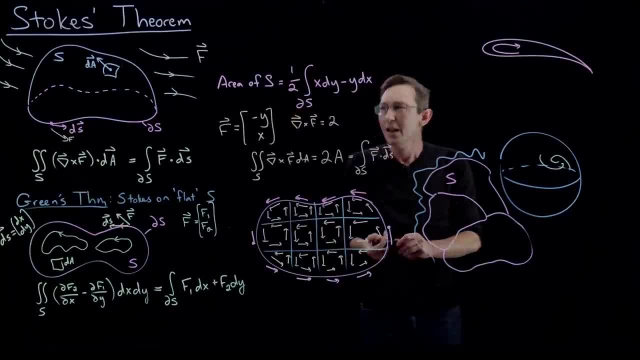 area of the parcel. so that's why I divide by 2 here. So long story short. if you want to measure the area of an irregular shape, you can just walk around the perimeter and compute this quantity along the perimeter of the surface.